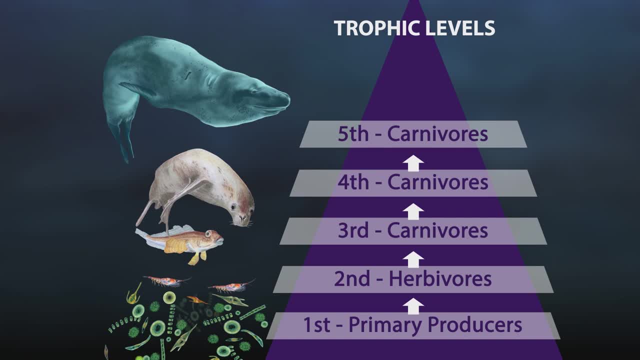 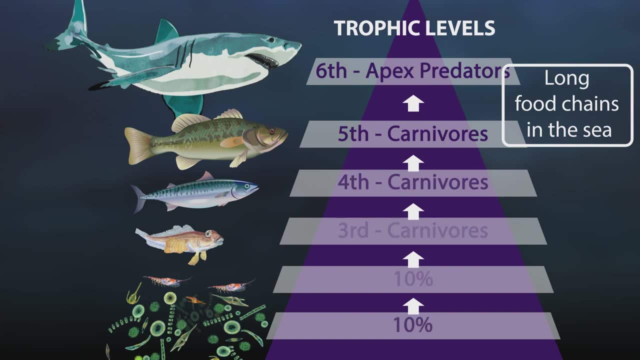 eat these tiny carnivores and in turn they are eaten by bigger carnivores. It's common for ocean food webs to have five or even six trophic steps, But as one animal eats the next, only 10% of the energy from the material they are fed on gets transferred up into the 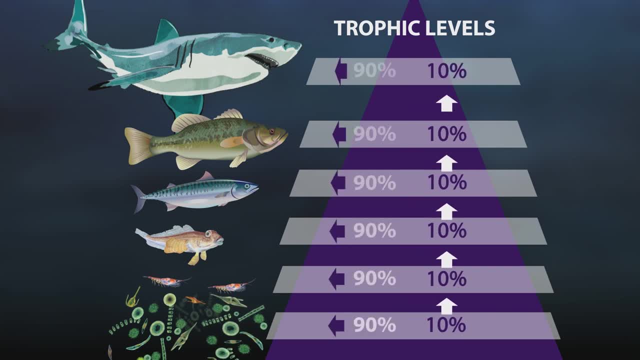 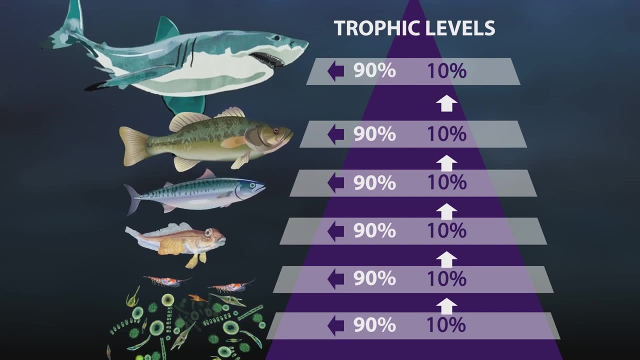 next trophic level. The rest- 90% of the biomass- is used by the animal to do all the stuff it needs to do: to grow, move, repair, or it's eliminated, it's pooped out, But here 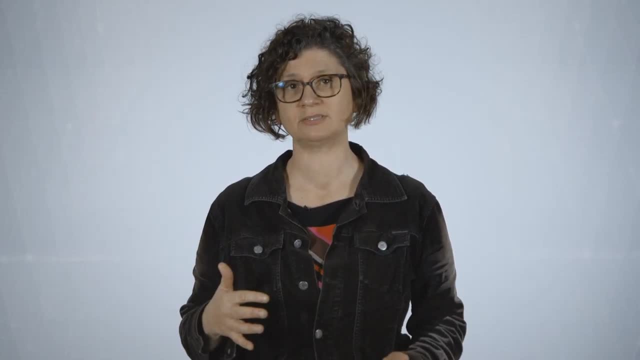 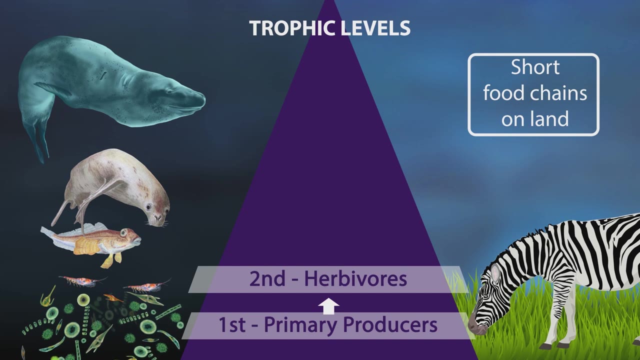 on land it's different. We have short food chains. Think about it. Plant material like grass and leaves are eaten by herbivores, and many of these are large animals, And then apex carnivores eat these herbivores. Sometimes you have other carnivores eating another carnivore. but many carnivores on land are first consumers, which means they sit only at that third trophic level. So on land food chains are typically short And long food chains exist, but they are rare. However, in the sea, marine food webs. 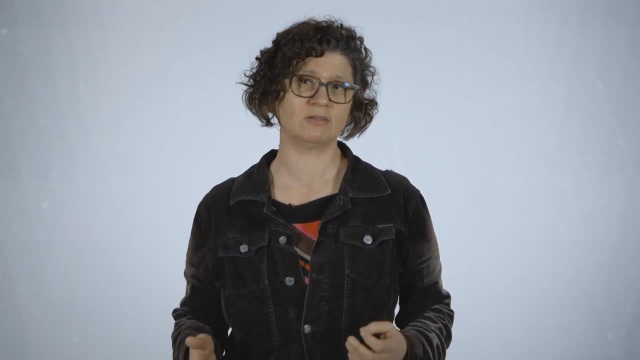 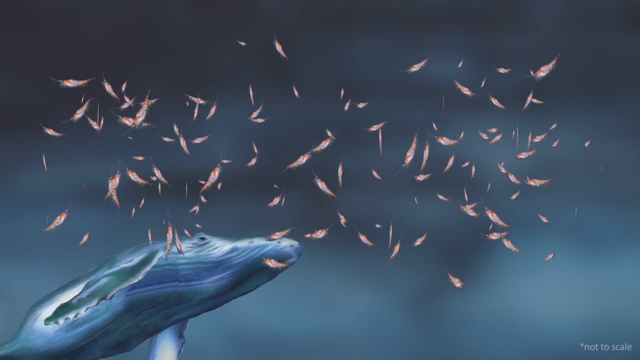 are extremely long, in fact the longest on earth. But it's not completely that simple, as the largest animals in the sea feed at low trophic levels. Huge filter-feeding animals like baleen whales strain tiny zooplankton from the water. We don't see the equivalent. 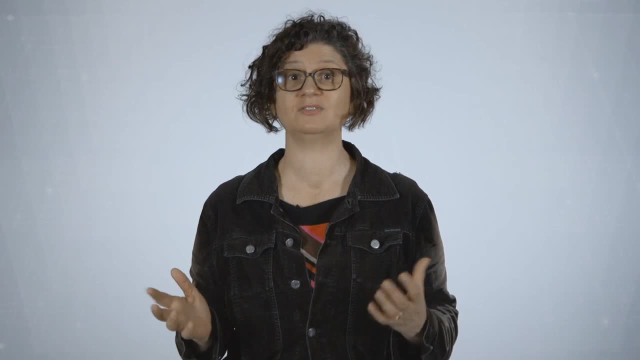 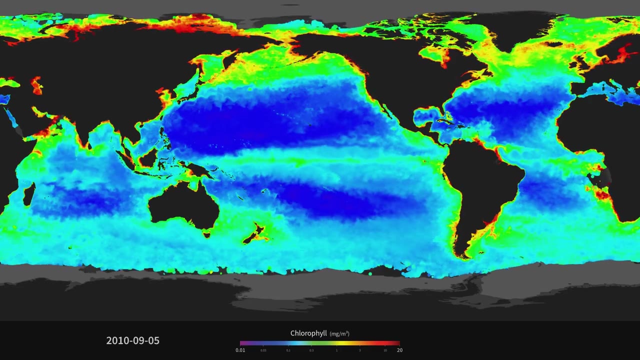 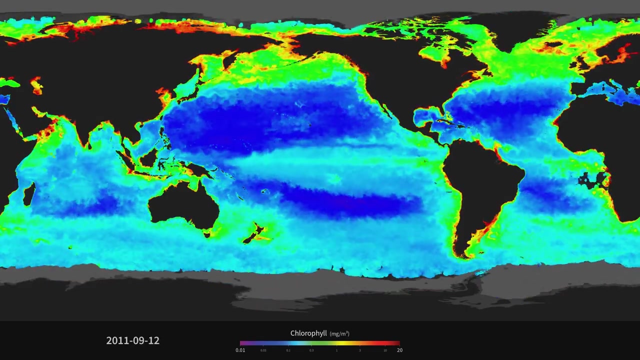 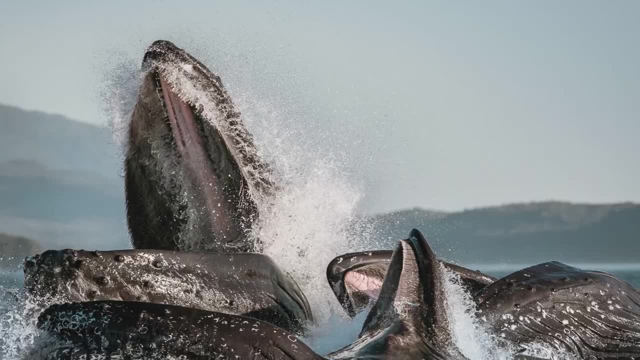 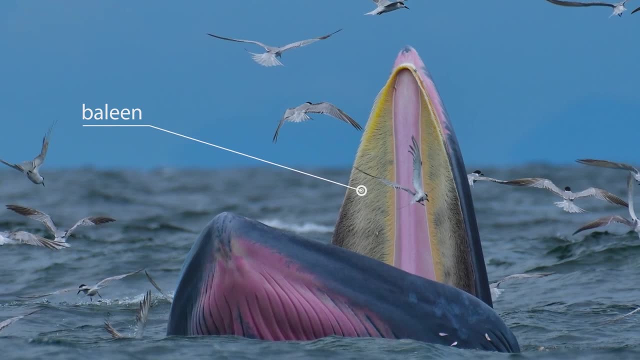 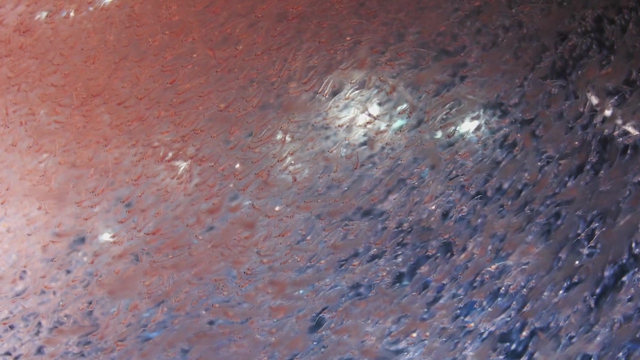 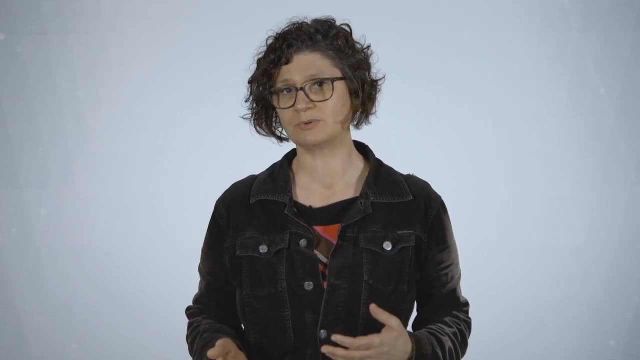 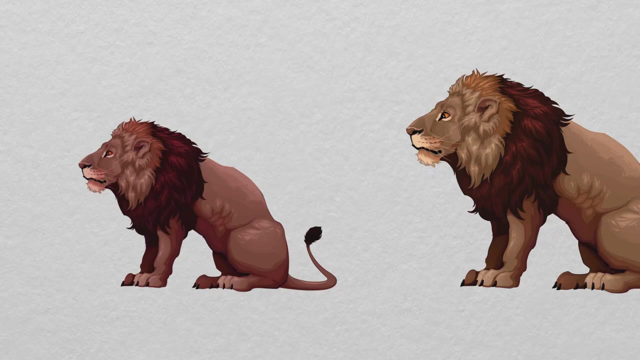 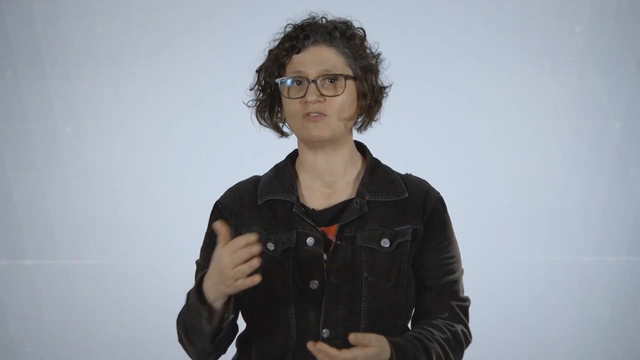 actually shark. well, you might eat shark fin soup. These fish sit at the top of the food chain, So eating shark fin soup or tuna is like us eating something that eats lions- that eats lions, if there was such a creature. So if we go back all the